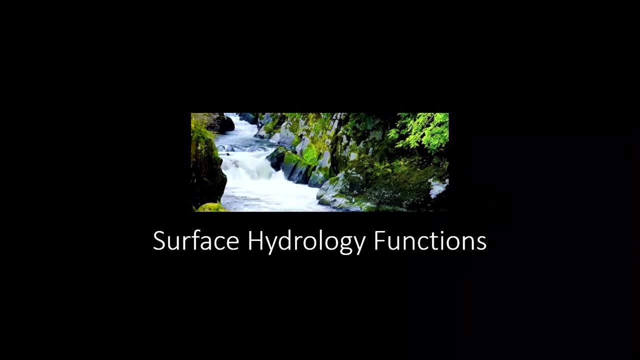 surface rasters. Typically, we'll use DEMs or digital elevation models to do this, with the z values depicting elevation, using the floating point grids instead of integers. In other words, floating points which allow for the potential for decimal points are not simply limited to. 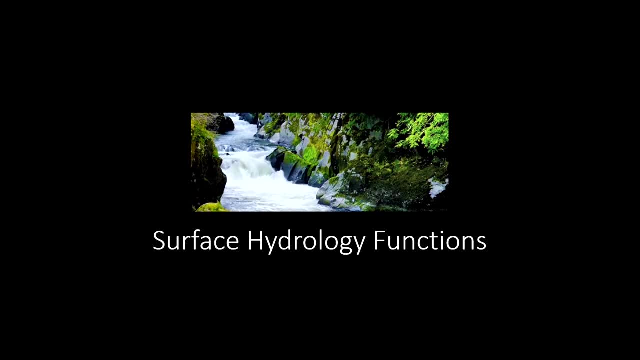 whole numbers, as is the case with integers. This allows us more precision in the processing of the data and the spatial functions that we're going to be using. But of course, we already know that, in general, integer grids are used to represent discrete data and floating point grids are used. 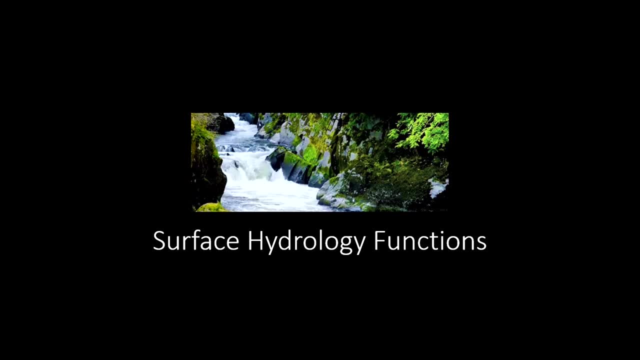 to represent continuous data, So we're going to use these to represent discrete data. and floating point grids are used to represent continuous data, So we're going to use these to represent continuous data. So we're going to use these to represent continuous data. Why I mention this is: 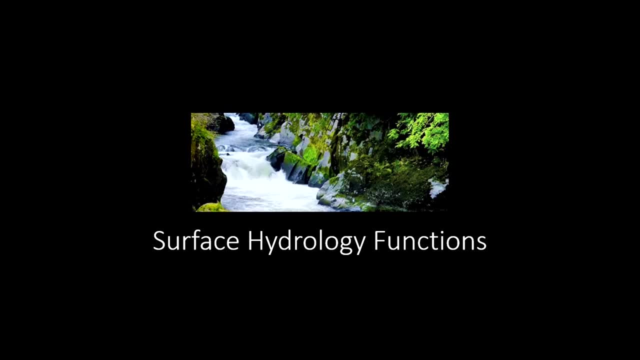 as we go through all of these different functions, we're going to have to kind of go back and forth by converting data from raster to vector. And why we have to do that is we have to keep in mind the limitations regarding the storage of the data, The surface hydrology functions that we'll be. 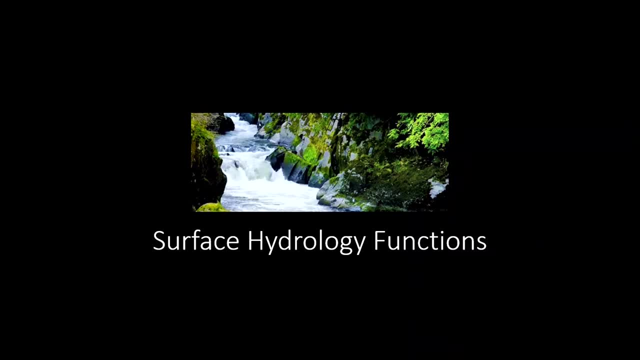 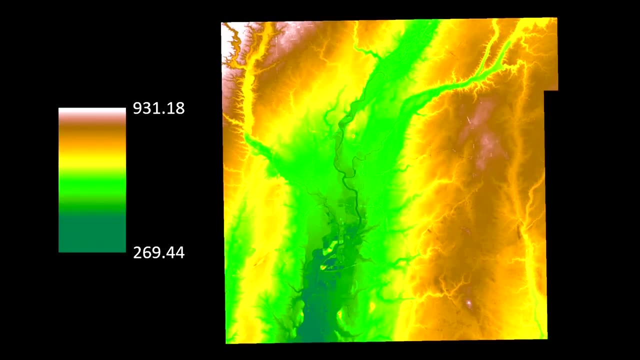 using include flow direction, sinks, fill, flow accumulation, stream network, stream order, flow length, basin and watersheds. Through our analysis, we'll be, for the most part, using this Marion County digital elevation model. This will be used as our input grid, but also later as our base map for our final output. What I'm about. 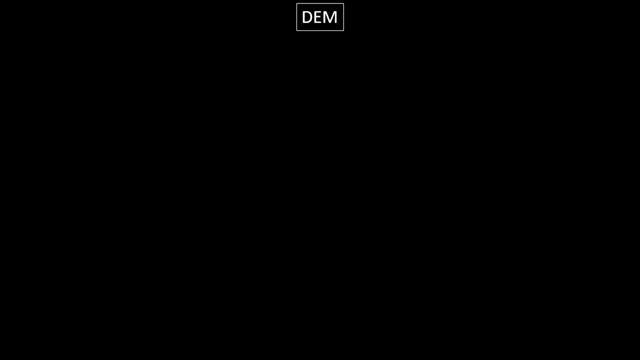 to show you is a modification of a flow chart that's out there. It's something that was originally created from ArcInfo, which then was replaced by ArcMap, which is then replaced by ArcGIS Pro, and who knows what's going to come next, But with a digital elevation model. 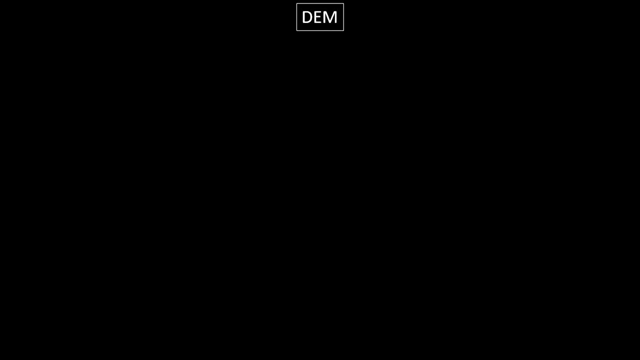 the first thing we would do is we would compute the flow direction, And we do that because the flow direction is going to help us determine the direction water flows across the surface. From that we can then help to identify or determine if there are any sinks. 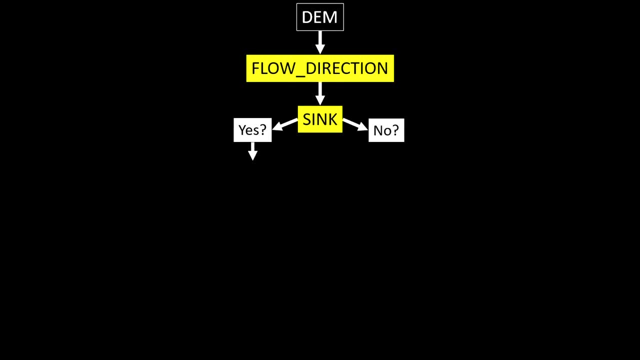 or pits in the surface. And if we do, if we identify that there are sinks in the surface, we got to do a little bit more to it. We got to fill those pits, We got to fill those sinks, And so essentially what we do is we then run a fill operation that fills those sinks.